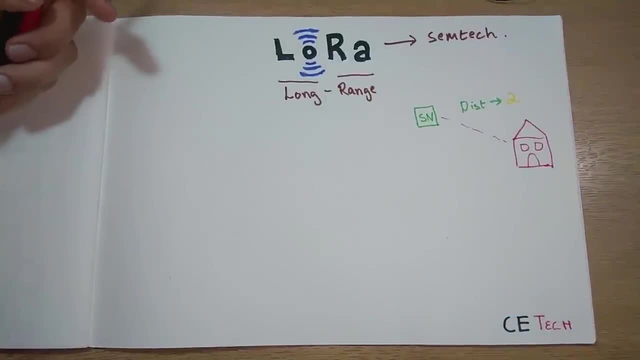 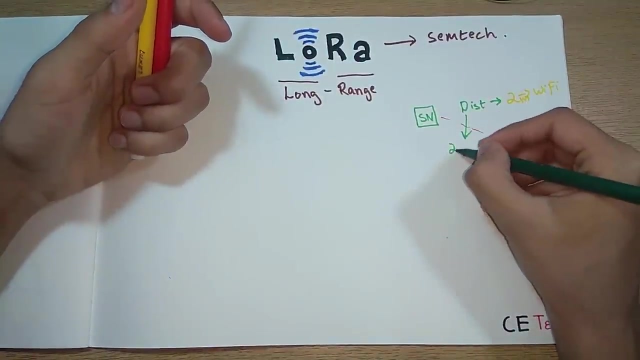 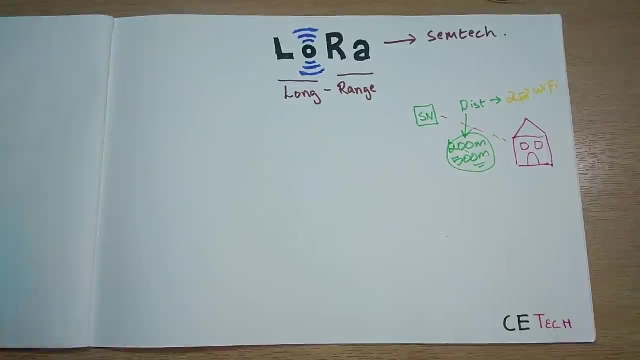 I device horrific meters, so it's like just in the outside of your house. so you might use Wi-Fi for this application? yep, why not? but what if I say that this distance is not two meters but is 200 meters or maybe 500 meters? what solution will you apply? you might use? you may say that you will apply. or you will add a GSM module to this and this will work for 200, 500 or any distance for that matter, because GSM, wherever you have the network coverage, it will work. so an alternative to GSM comes in LoRa. there are modules available like this for LoRa. you will just connect LoRa to the sensor. 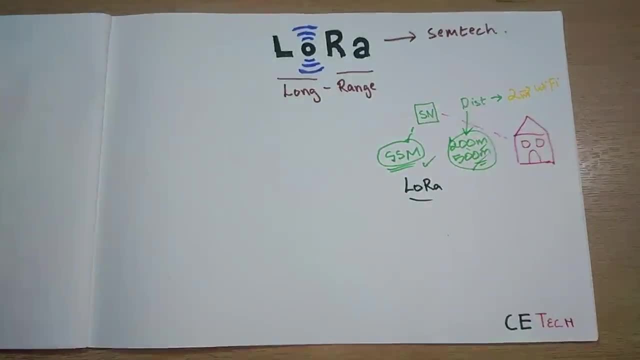 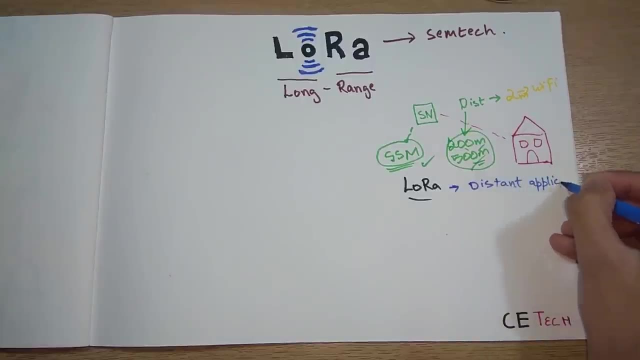 node and you will also add one LoRa over here and that will do the work. I will tell you more that how LoRa works, but LoRa is very useful in distant applications where the distance is large and the data that has to be sent is less. so one good feature is that you can achieve very large distances: 500 meter is very. 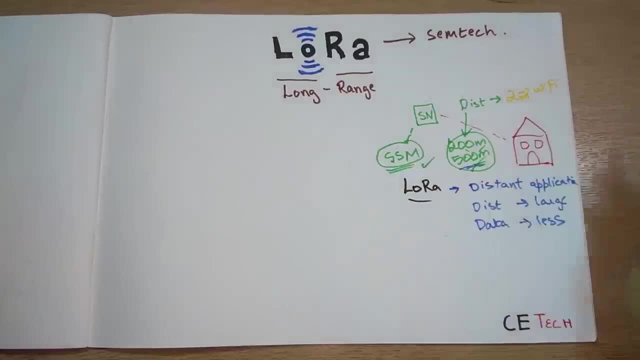 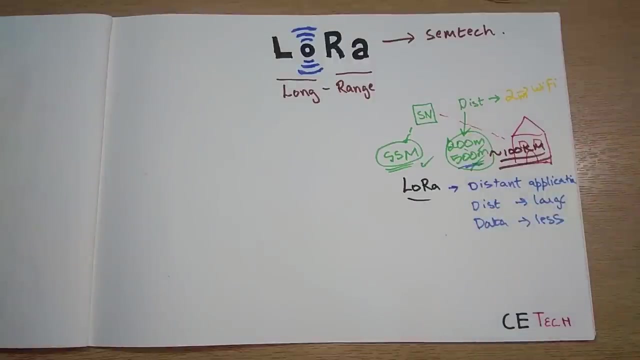 easy. if you use a better antenna, better line of sight and things like that, you can achieve distances to up to up 200 kilometers. yes, that is correct, you can achieve distances up to 100 kilometers with LoRa, so, but the disadvantage is that you need to use less data. you need to send less data at one time, so talking. 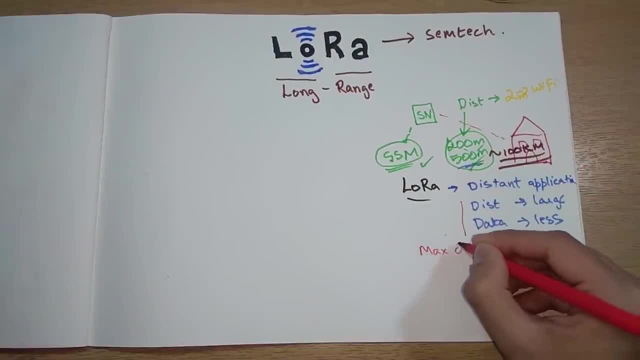 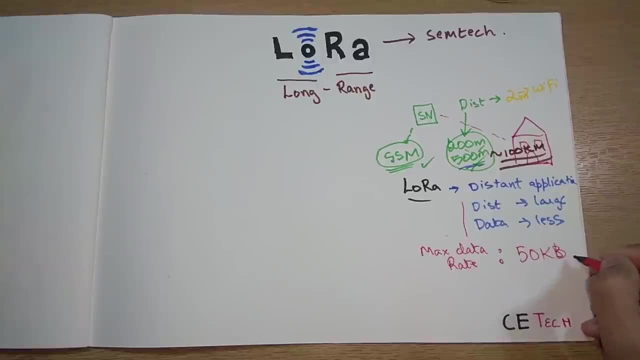 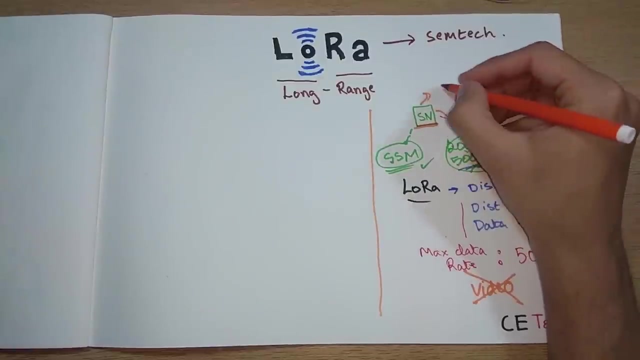 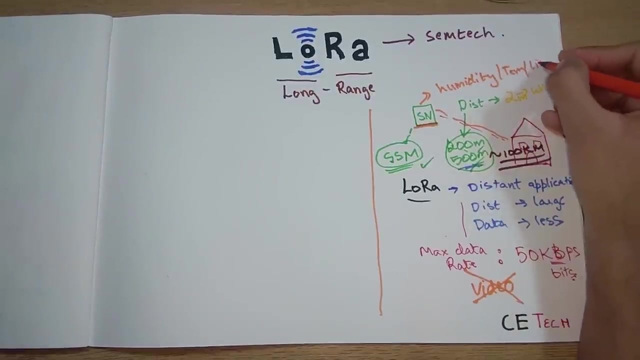 about data. the maximum data rate for LoRa is 50 kbps- sorry, kbps, so this is bits. so things like video transmission is not possible, but what is possible is transferring sensor data, so this: so sensor may be a humidity sensor or a temperature sensor or a light sensor, whatever it may be, so this type of 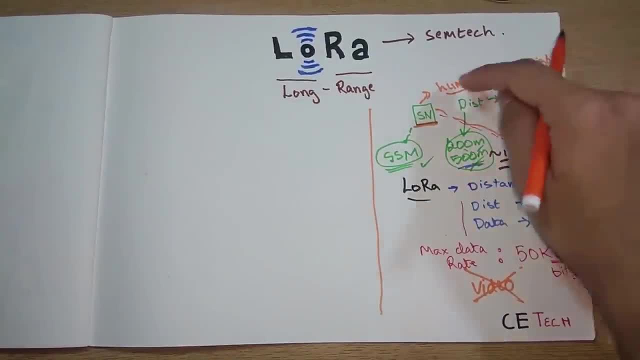 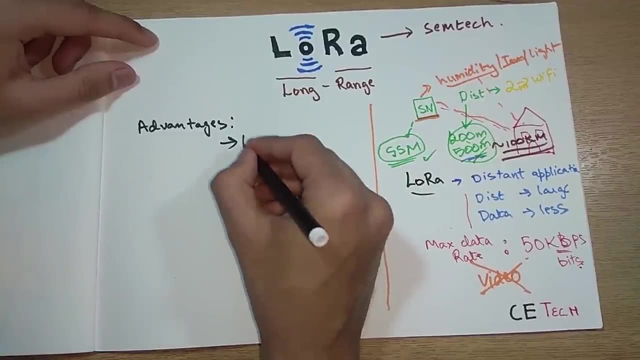 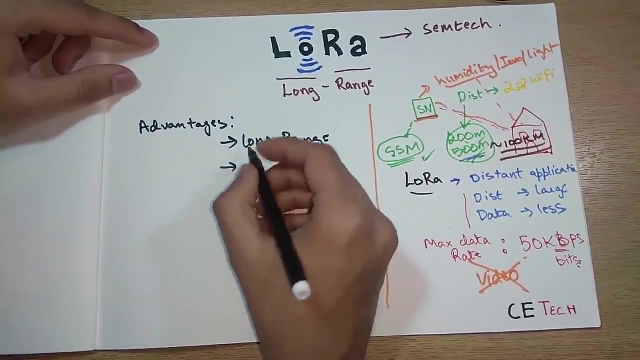 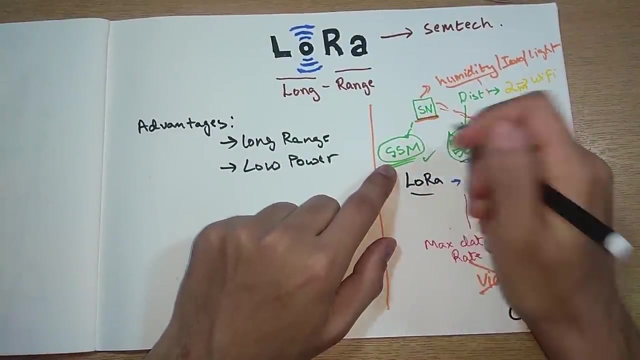 data doesn't change very rapidly in certain conditions. so there you can apply LoRa. so now talking of the main advantages, it is long-range also. one thing is you can achieve very good battery life out of this, so low power also. so where you can use GSM as well- GSM or 4G or any of that. 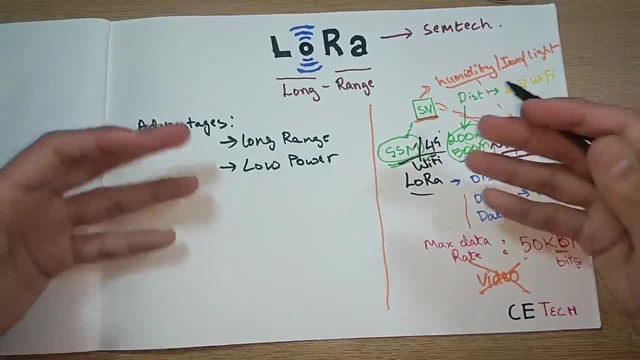 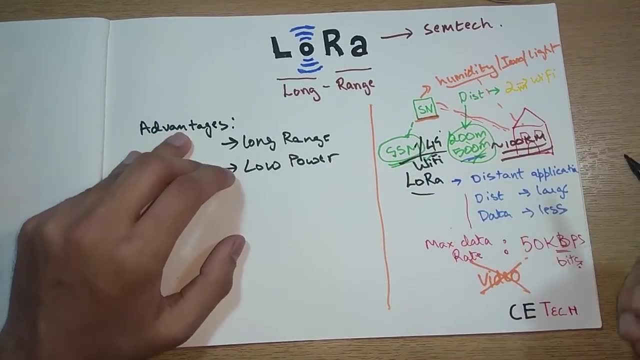 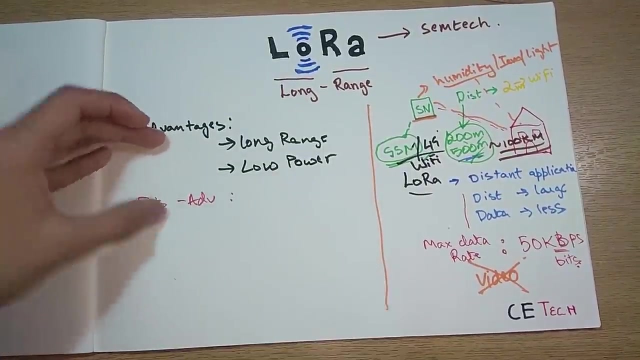 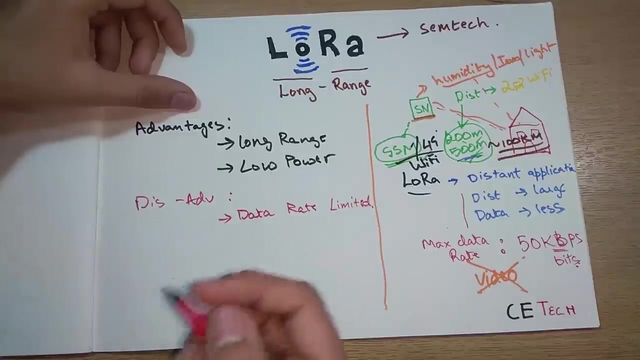 thing, or Wi-Fi consumes a lot of power. LoRa consumes a very little power, like 10 milliamps, 20 milliamps max, while transmitting or receiving in certain modes. well, the disadvantage for LoRa is that the data rate is limited. so by saying, 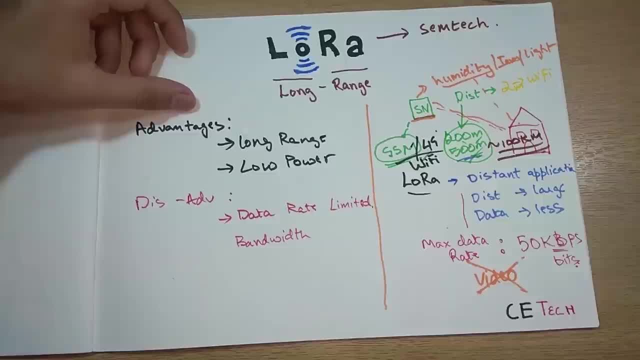 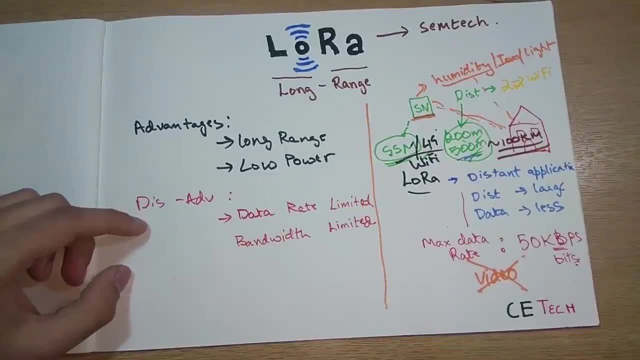 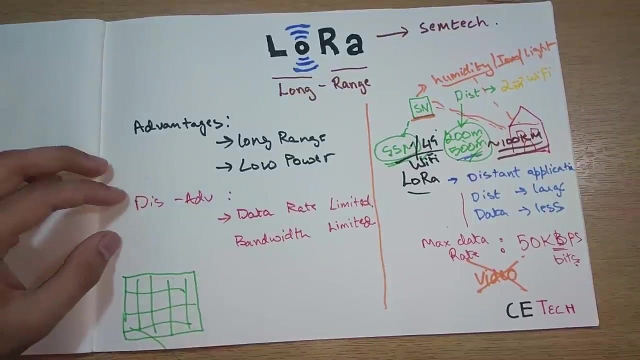 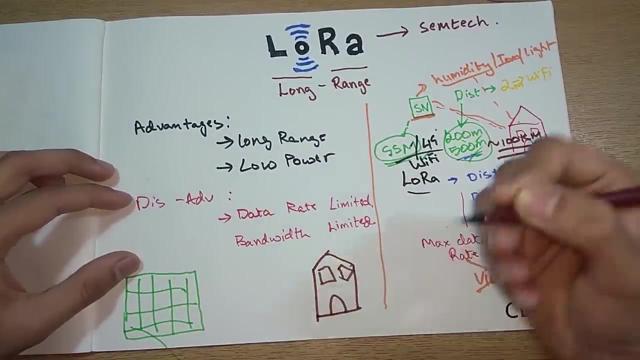 this I say that the bandwidth is also limited. so, taking a typical application of this, so suppose I have a farm. so there is my farm. I represent it by green color and I have a home which is far from my farm. again, a poor drawing of my home and 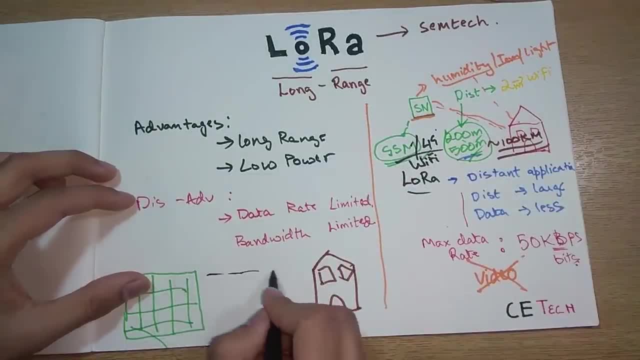 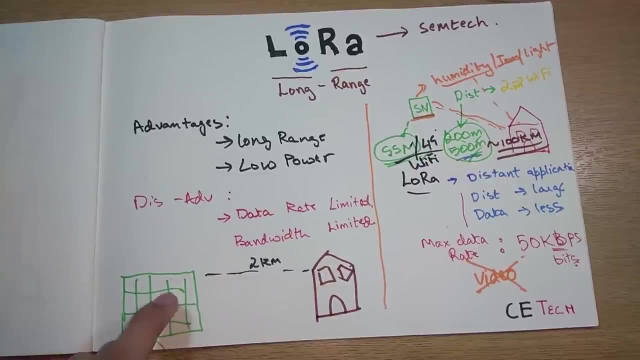 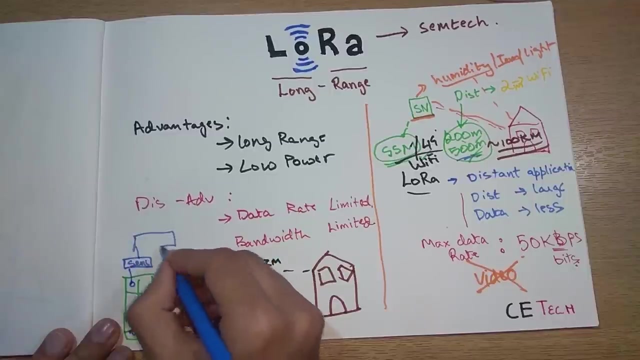 the distance is like, say, two kilometers, and I need to see, I need to monitor humidity at all times of my farm for four different points. so what I will do is add a humidity sensor connected to Laura and we'll all use, obviously, a microcontroller and add a battery for it. now this Laura will be connected to a. 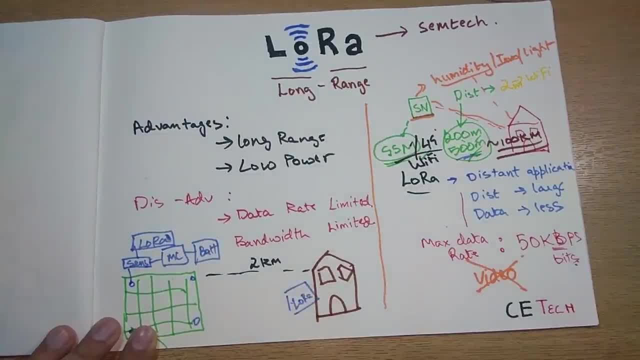 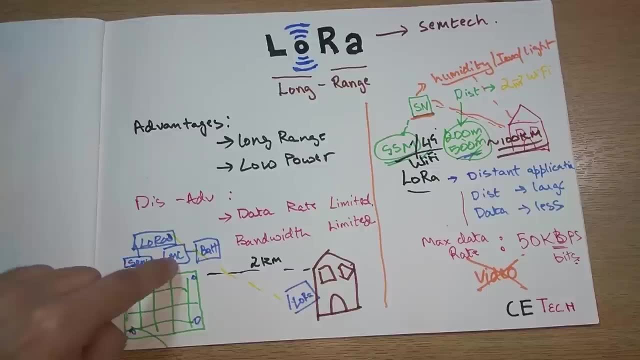 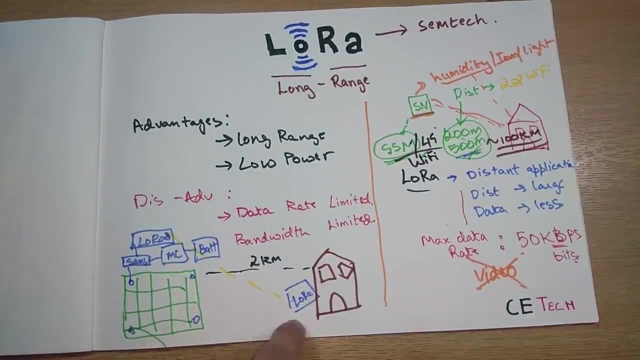 Laura at home. now, in this case, Laura is low power consumption. microcontroller can be connected to a microcontroller at home. so I am going to connect to a microcontroller at home so I can go to sleep after taking consecutive readings like every one minute or every two minutes or whatever the use case is, and 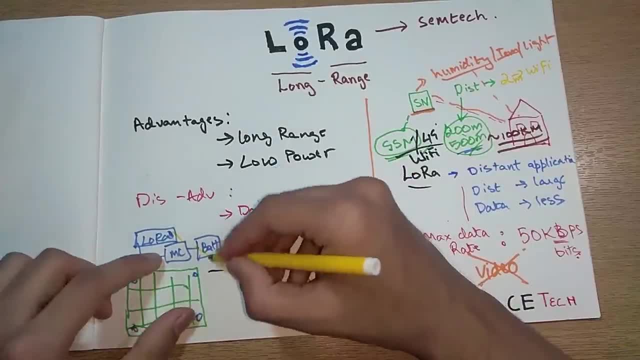 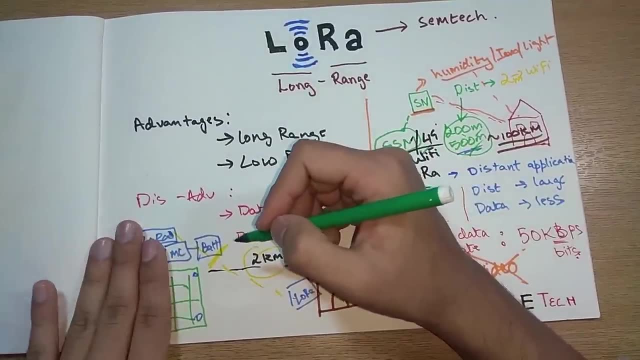 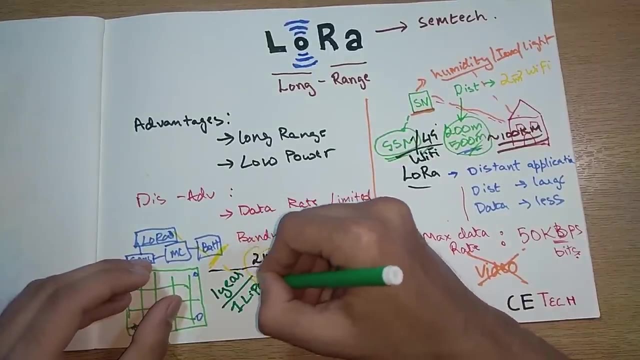 we achieve a good distance, we can power this entire system with batteries and we can also achieve a good battery life. that is, this entire system can be entirely powered by batteries up to one year- yes, one year, with a one lipo battery. these tests have been performed. distance tests have been performed. 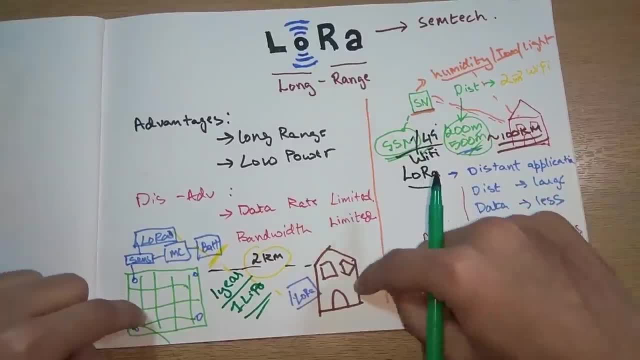 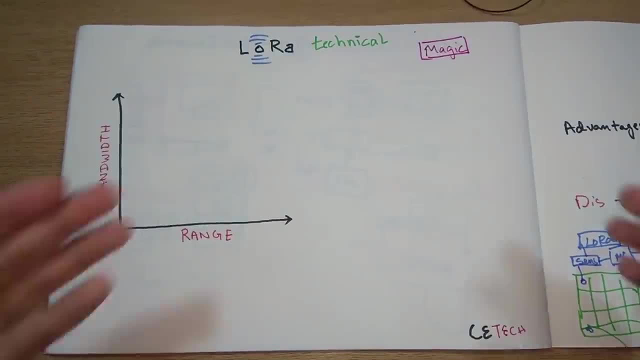 battery life has been performed, so this is very much applicable in situations like this. now moving on to the technical aspects. so you might ask: that is LoRa magic that it does so long distances and it does not consume power? how can it do that? no, it is not. 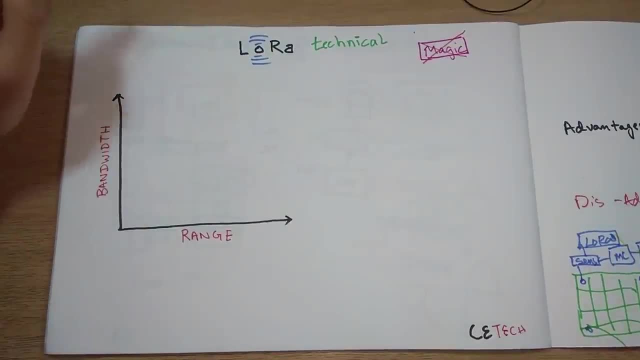 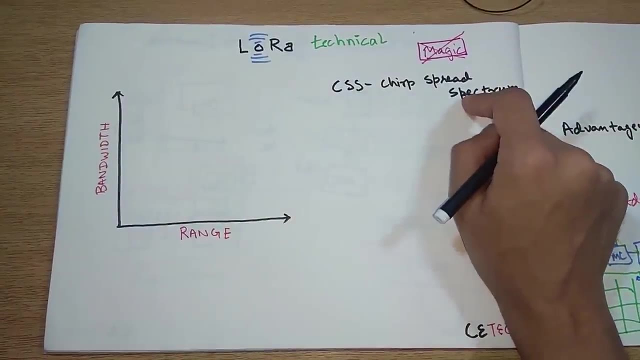 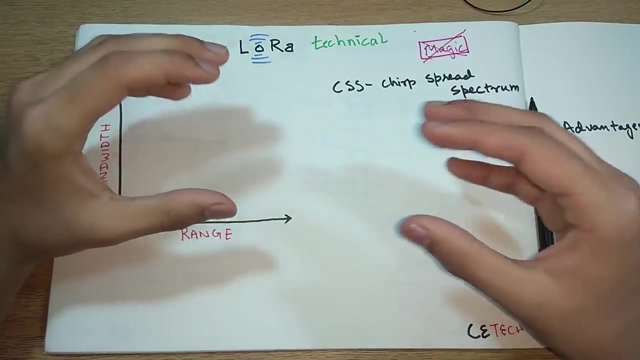 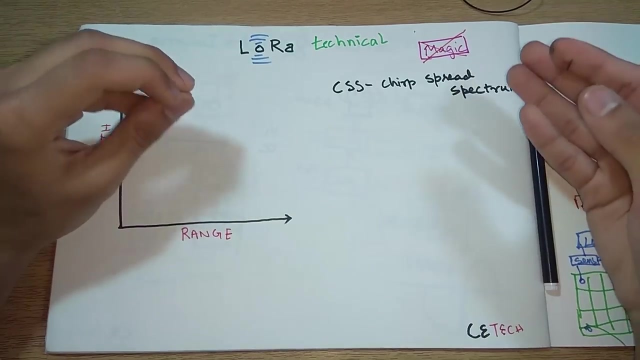 magic. it is pure science. I will tell you the science behind it. the main thing behind it is CSS. CSS is chirped spread Spectrum, so this is a modulation technique. what modulation is is the signal that you have is changed in such a way that it gives better features. 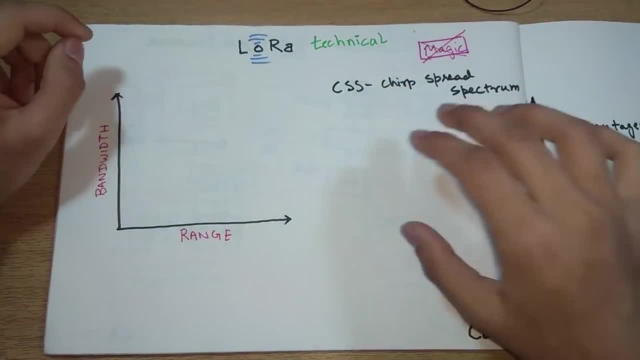 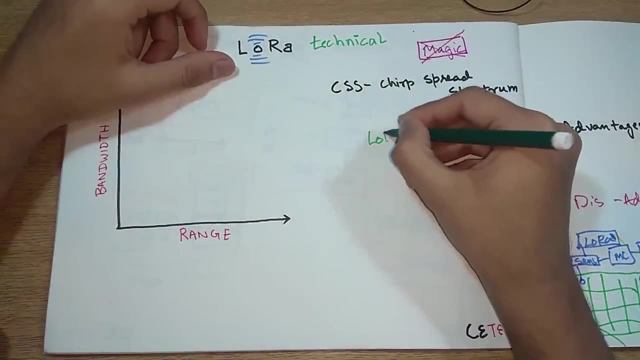 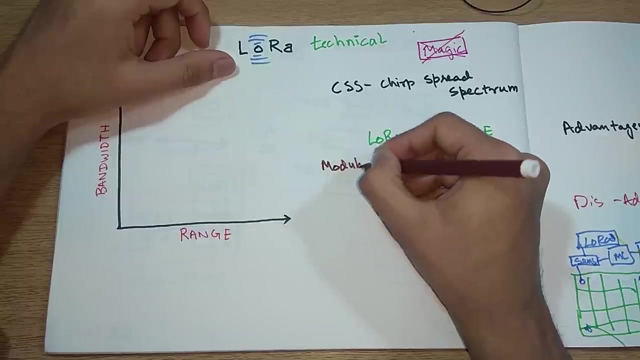 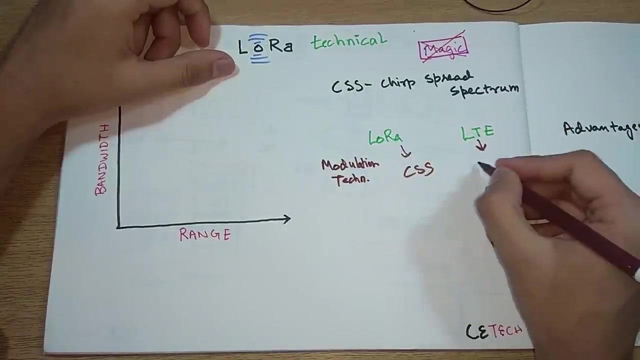 so chirp, spread spectrum, or CSS, is a modulation technique that is mainly used for LoRa. for better understanding, let's directly compare LoRa with LTE, so that the first thing we will see is modulation technique. so LoRa uses CSS, as I told you, and this uses FDMA. FDMA is frequency division multiplexing axis. 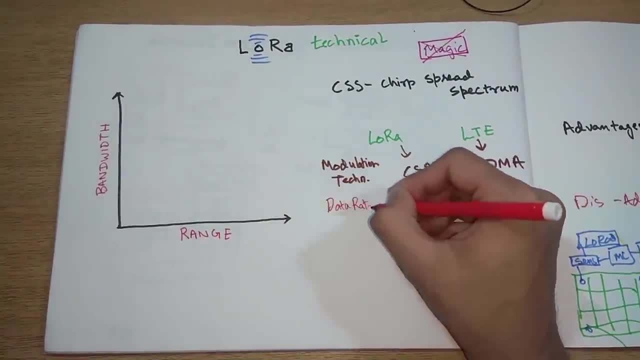 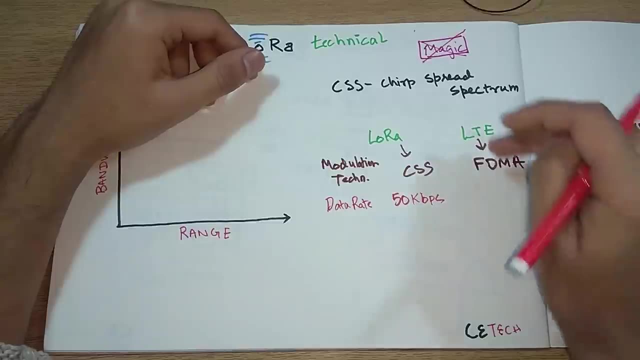 the second thing we will see is data rate. the maximum data rate we can achieve with LoRa is 50 kilobits per second, while LTE is much faster. you can stream videos etc. but LTE is much faster, you can stream videos etc. but LTE is much faster, you can stream videos etc. 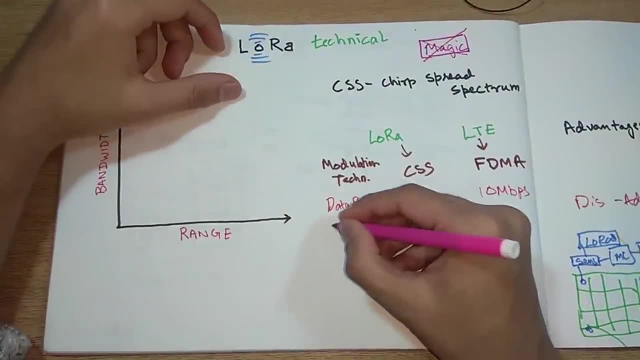 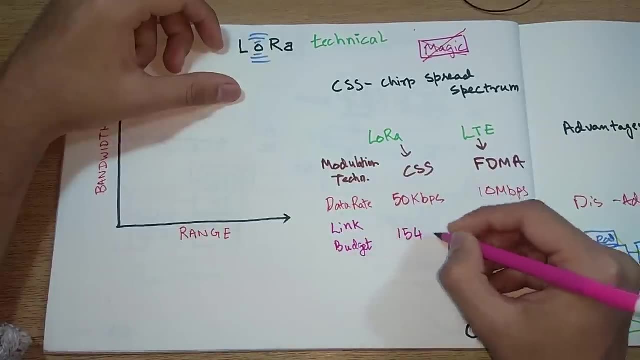 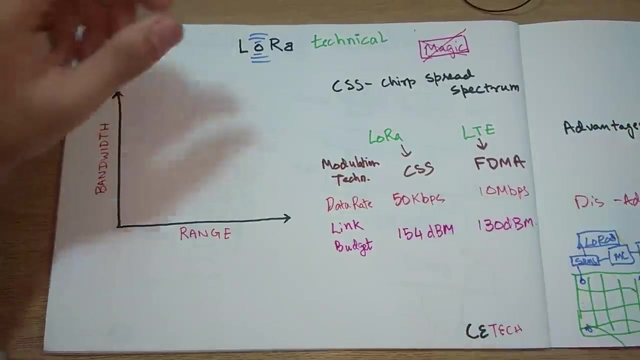 but LTE is much faster. you can stream videos, etc. with 10 Mbps. one technical term is link budget. link budget for LoRa is around 154 dBm, while link budget for LTE is around 130 dBm. you might ask what is link budget? yes, I will tell you that link budget is just like pocket money. 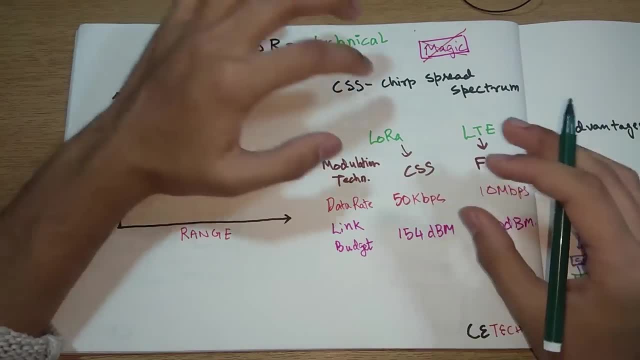 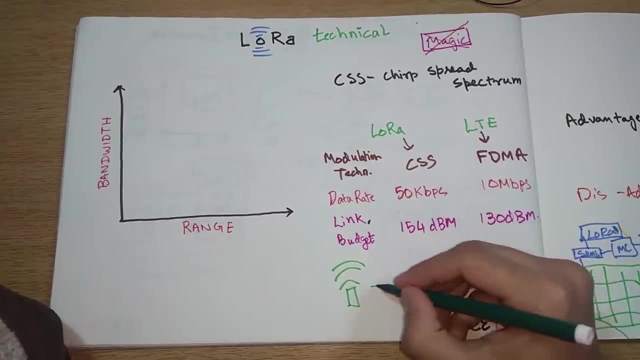 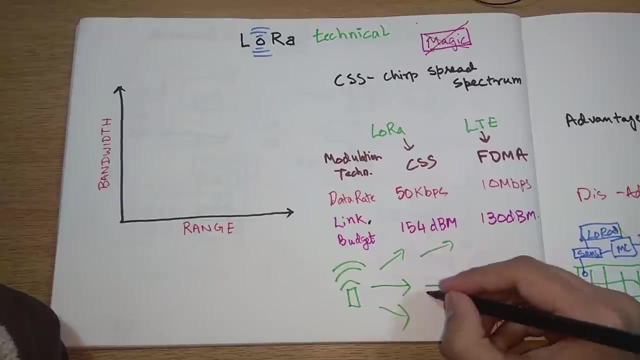 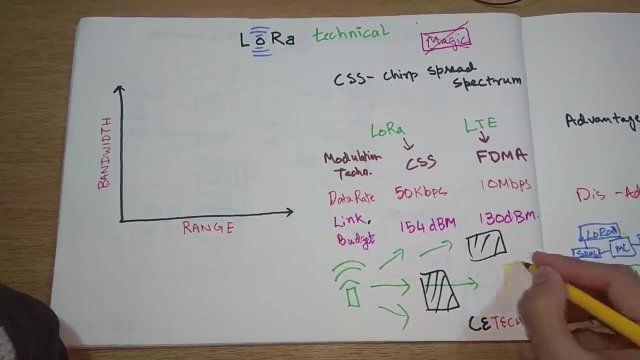 the more you have, the better. so in this case a link budget. say, suppose you there is an antenna transmitter over here. this will radiate signals all over the place and there will be things in between, so there will be blockages and your trans and your receiver will be at a far distance from the transmitter. so 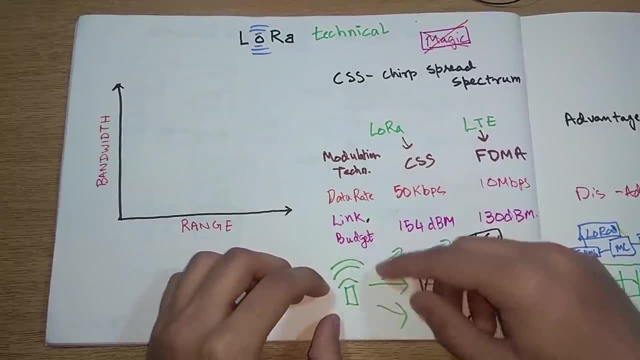 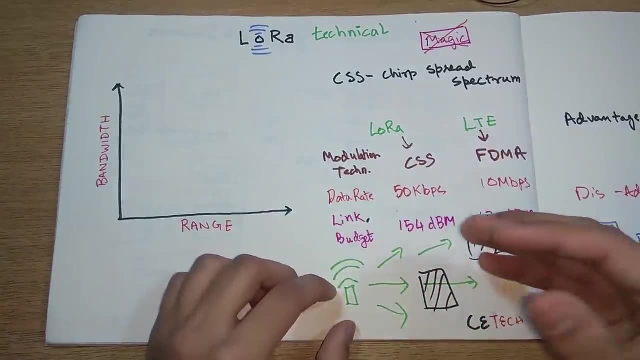 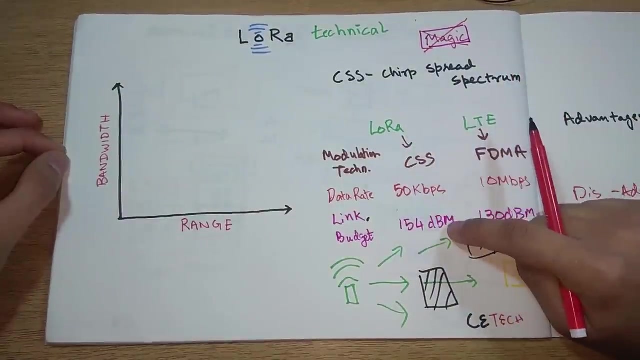 more the link budget of the signal or the technology or the modulation technique that is used in this antenna while transmitting the signals, the better the capability of that signal to reach reach at the receiver. so according to that explanation, you can obviously understand that as laura has a better link budget than lt it has, it has definitely a better range. 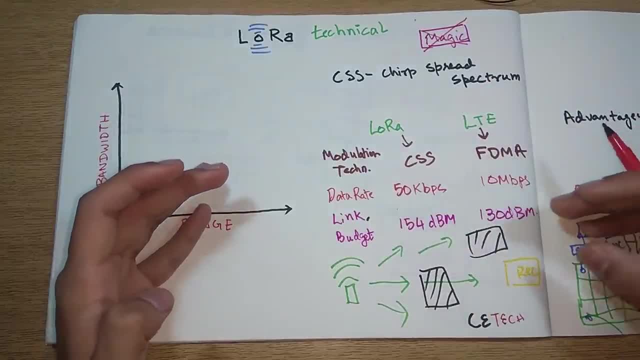 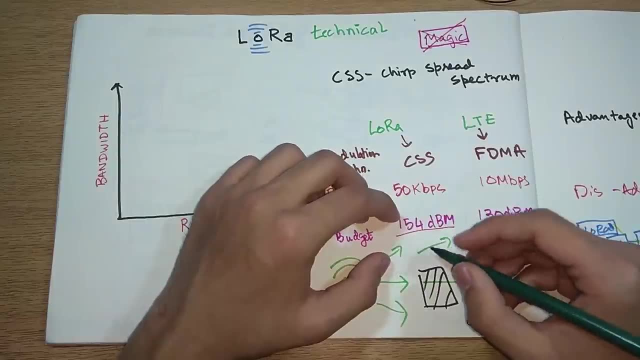 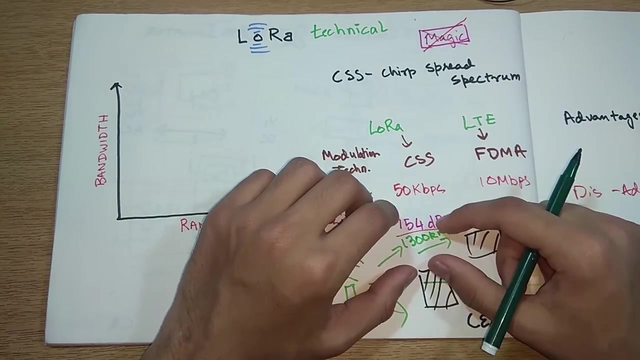 and a better capability of transferring signals. with this link budget and taking ideal conditions, we can calculate range to be around 1300 kilometers. but as this is ideal case, uh, there are many attenuations that happen in the wire that is used in transmission and there are blockages in between. 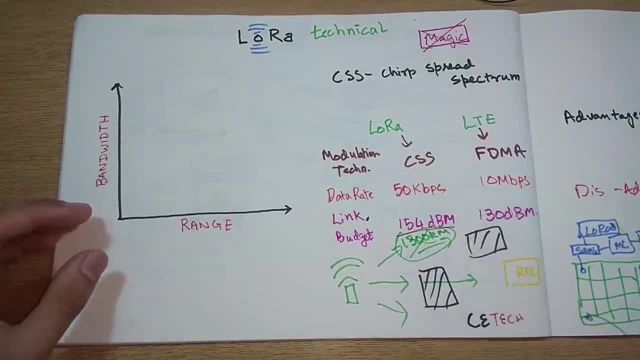 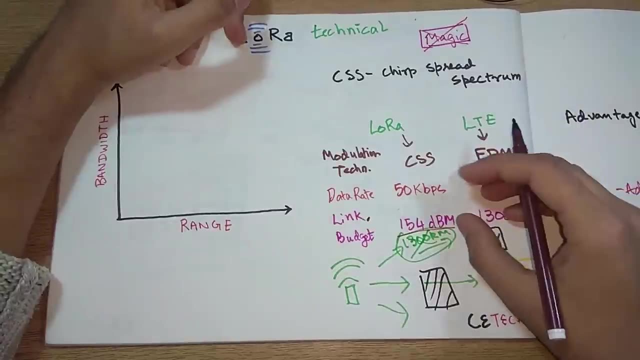 etc. etc. so we do not get this range, because this is ideal. we get a lesser range, but this is a very good link budget that we get for a such a cheap price. so the main trade-off is the data rate, and data rate is directly uh, uh. 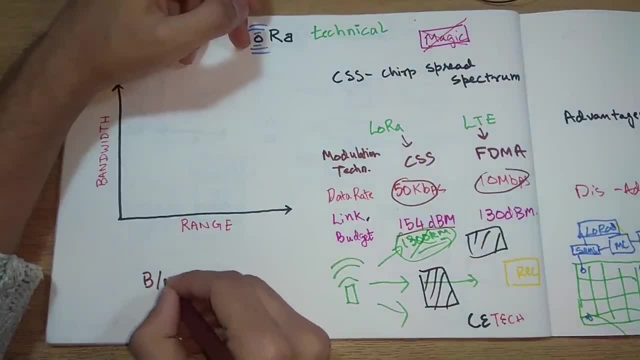 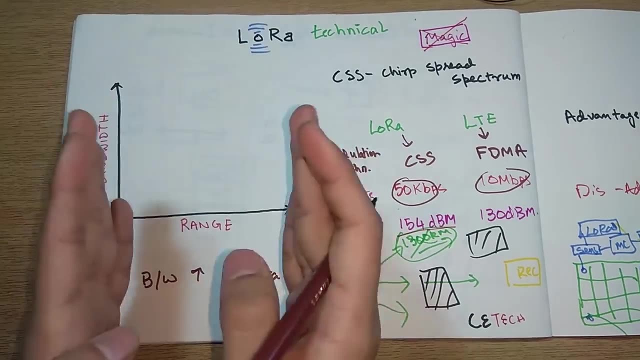 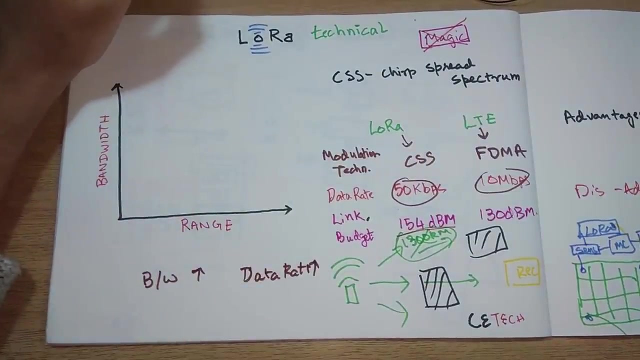 linked with the bandwidth, so more the bandwidth. so i'll abbreviate the bandwidth with vw, so more the bandwidth, lesser, more the data rate. the bandwidth of the channel is the amount, the amount you can send at one time. so here i have a bandwidth versus range chart where i will use 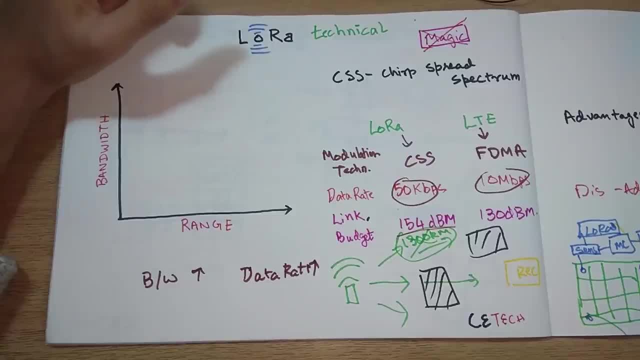 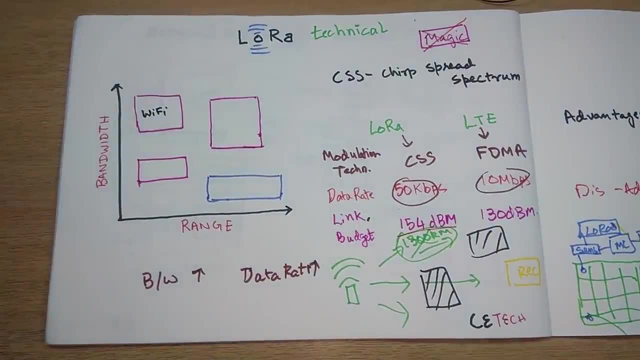 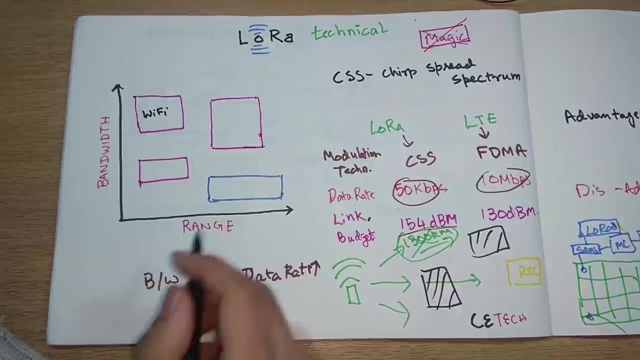 which i will use to compare different technologies. so here i have made four boxes which i will fill out. the first one is wi-fi, the most popular for makers in iot. so wi-fi has a very high bandwidth. you can obtain very high speed uh internet connections using wi-fi. 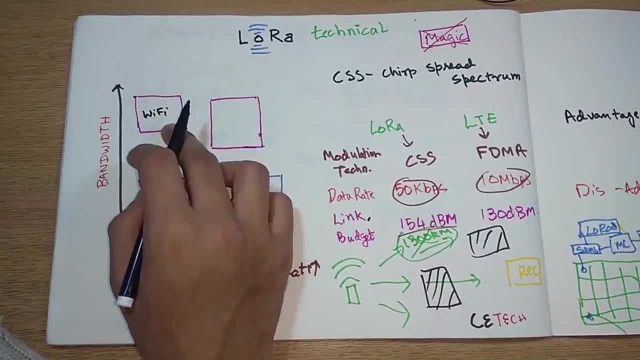 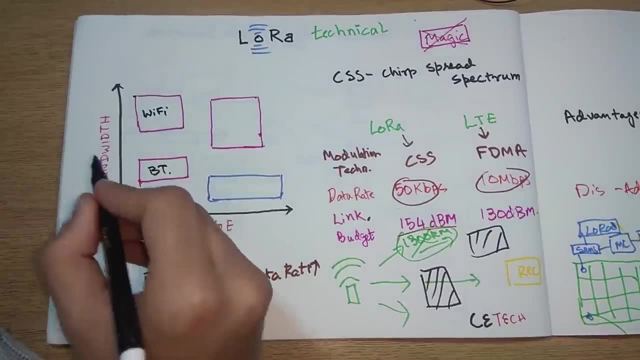 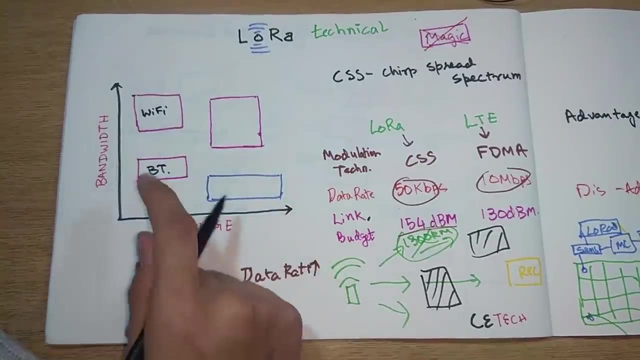 but the range again is too small for wi-fi. on the other hand, for the same range we have bluetooth. so bluetooth but has a lesser bandwidth. you cannot stream videos with it. maximum to maximum you can stream audio with it. that also medium quality, this box with a good range and a good bandwidth. 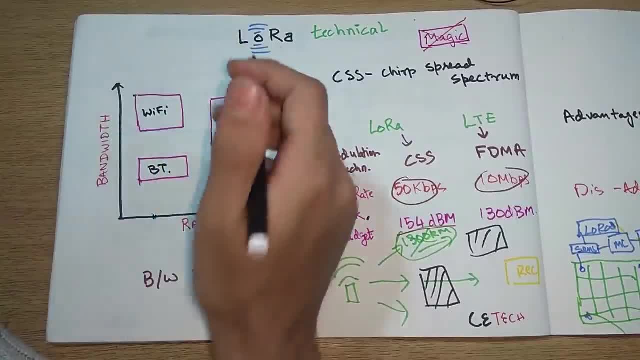 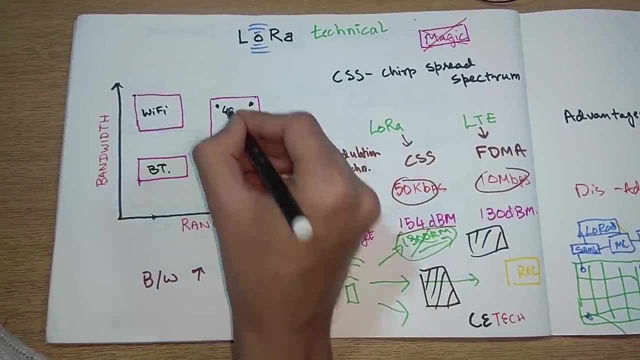 is 4g- lte, gps- and it has a very high bandwidth so you can obtain very high speed internet connections, gsm, etc. so on this side, with higher bandwidth on this side and on this side. so this will be 4g, this will be 2g and all mobile networks basically, but this box is the special box that we are. 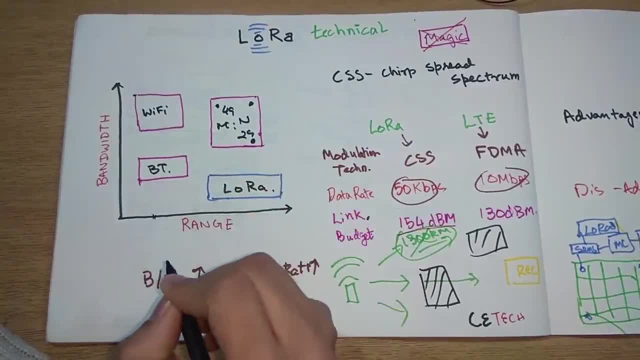 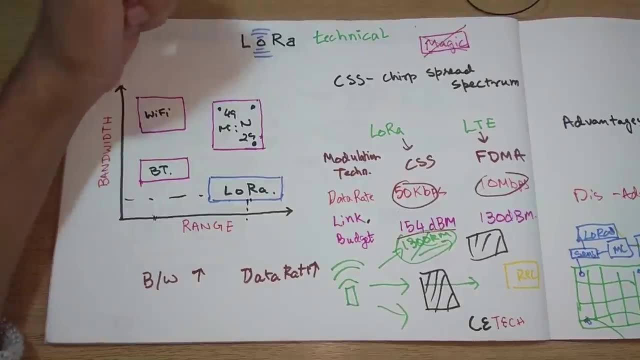 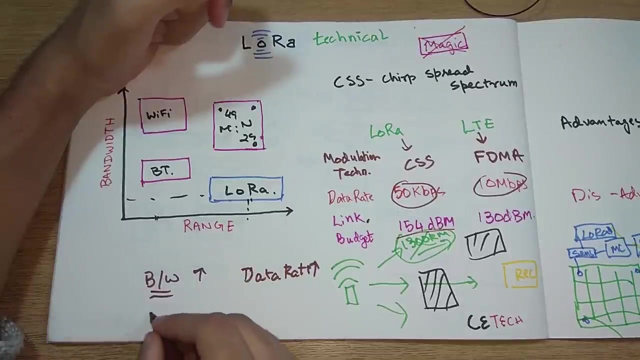 studying about this has laura in it. so what laura can do, it can provide very high range, but for a low bandwidth. so in laura you can also play with the bandwidth, so you can select your bandwidth and according to the bandwidth you can change the range. so if your bandwidth, if you increase your 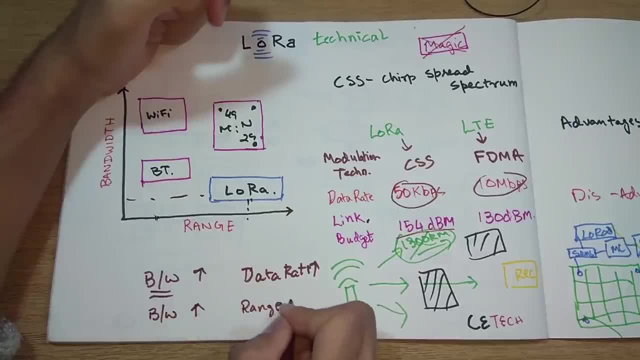 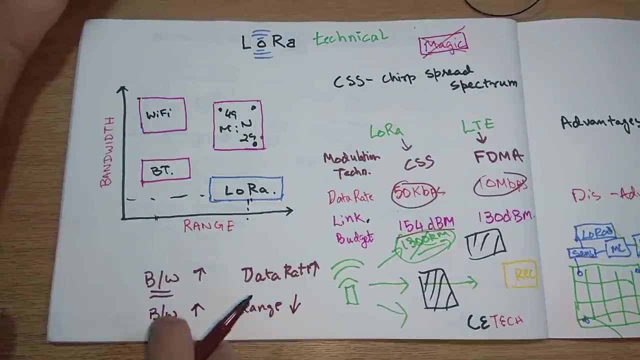 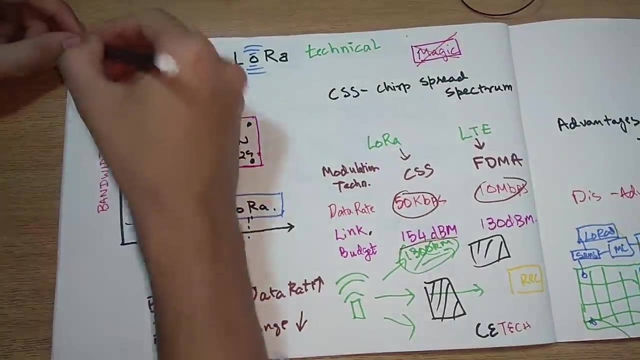 bandwidth, your range decreases, so you can select your bandwidth according to your range. but selecting the bandwidth is a special case, as you need to see how much data you need to send and according to that you need to select your bandwidth. apart from this, you might have heard 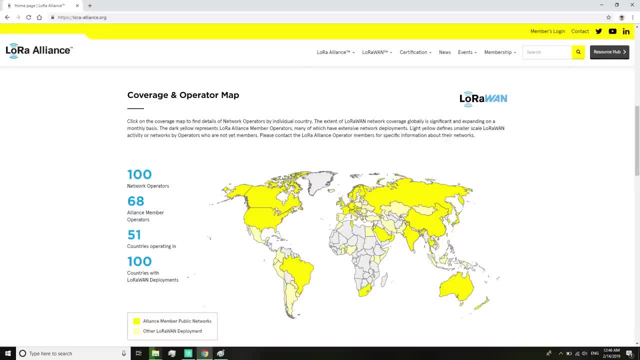 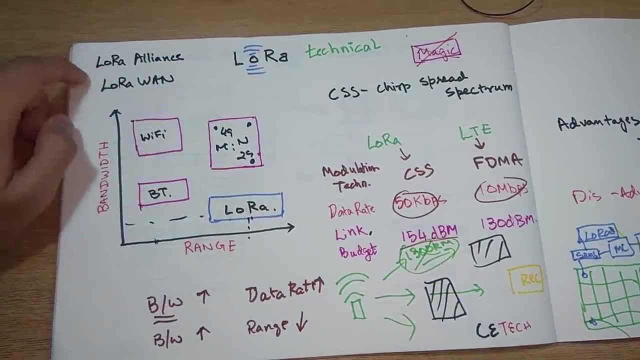 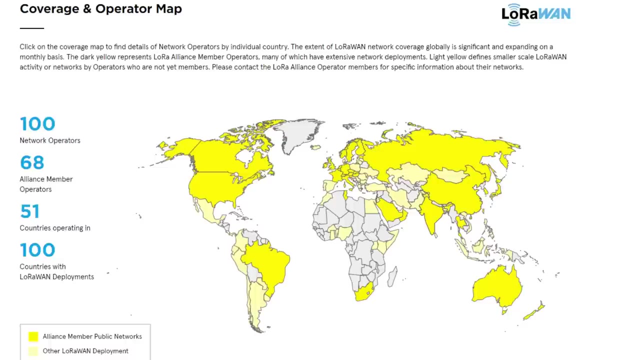 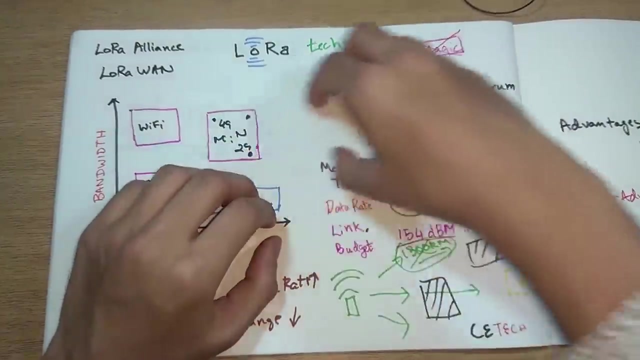 about laura alliance and laura van. these are two terms that you also need when learning about laura. so laura alliance are the set of the companies, or many companies, which support laura and which use laura and they have networks for laura. on the other hand, laura van is a laura network which is spread over a wide 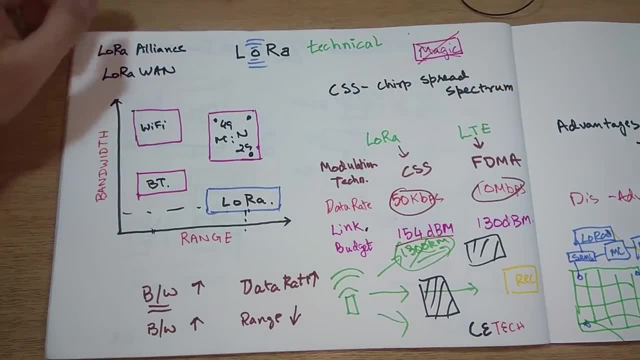 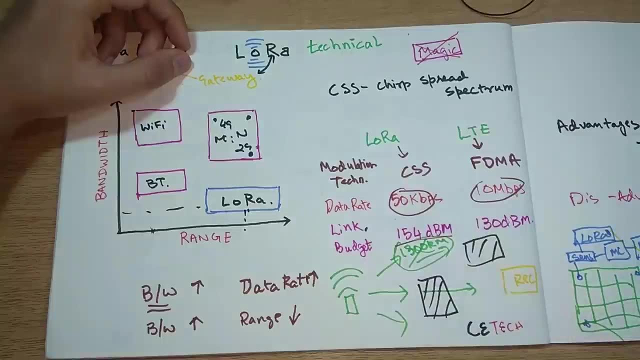 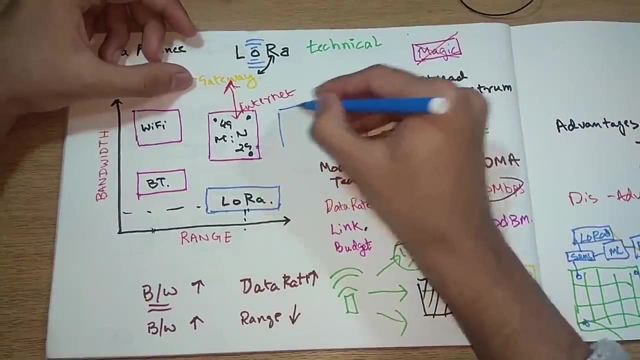 area. so this happens using a network which is spread over a wide area. so this happens using a LauraVan gateway. so what a gateway does? it connects Laura with 4G as an internet if you have a big area. so this is like, say, a hundred kilometers by. 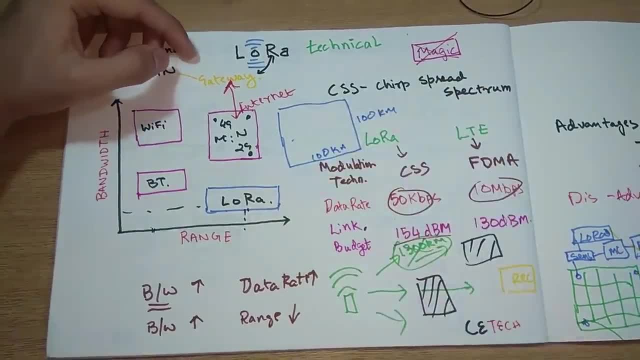 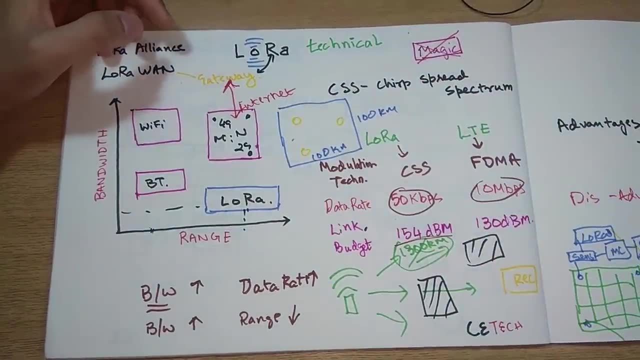 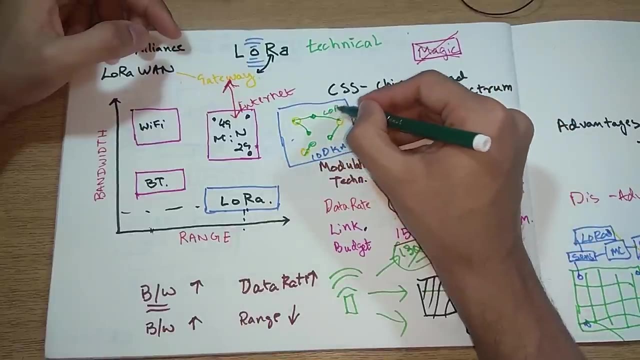 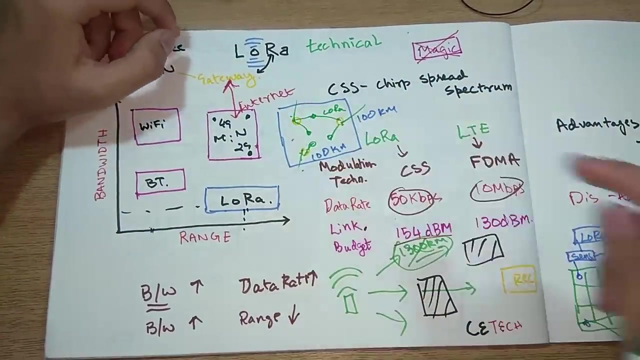 hundred kilometers. so we will have Gateways. so we will have Gateways, some, some somewhere here, here and there, And all the sensor nodes will connect to these gateways using LoRa technology, and these nodes will be connected to internet directly. These are like base station towers in mobile networks, So these will connect to the internet and all the data from the sensors will be directly uploaded to the internet. 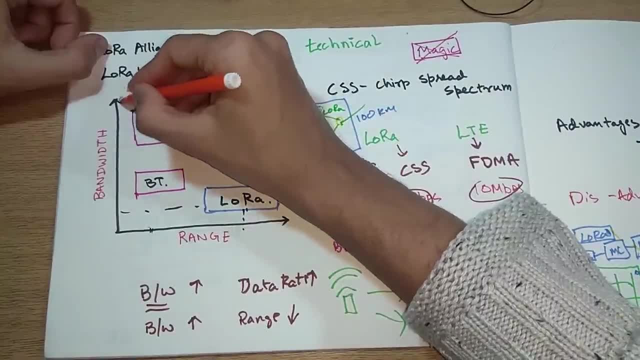 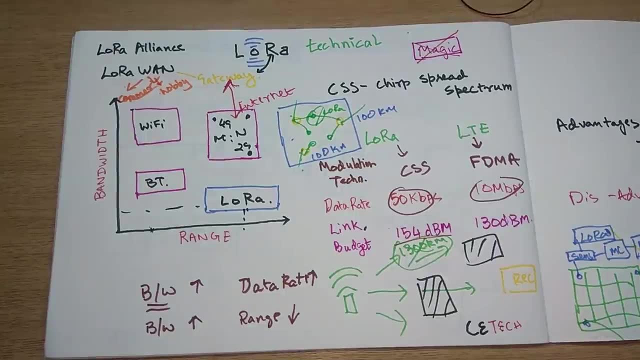 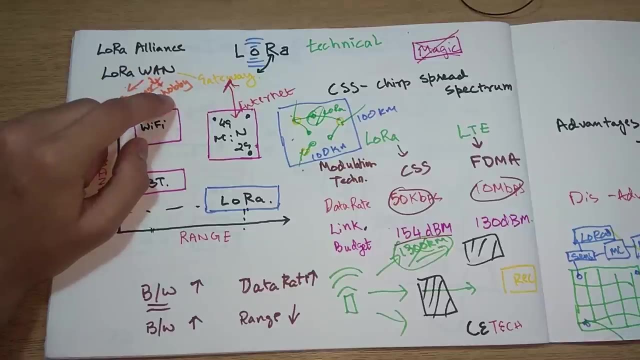 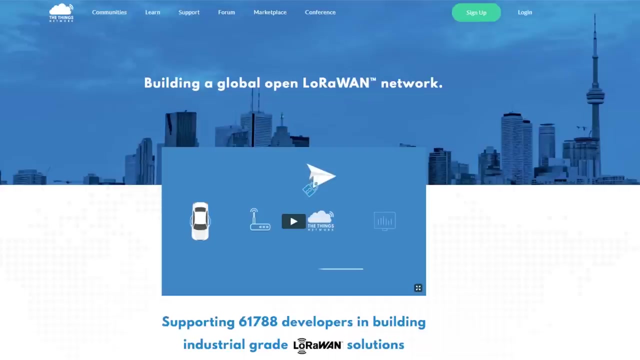 Now, these LoRaWAN gateways can be applied to two types. It's commercially and hobby style. So commercially, companies use this to run their products, to transfer data to their products. According to hobby wise, or you may say community wise, you can use LoRaWAN using a site called the things network. 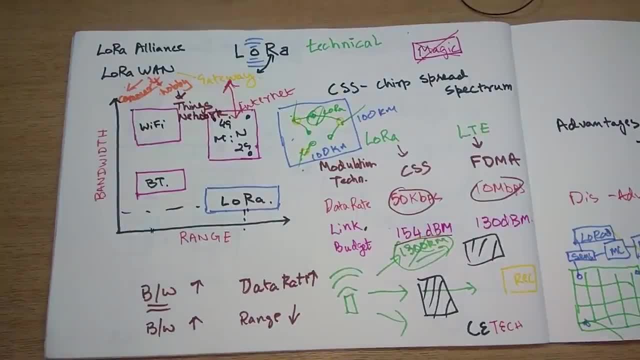 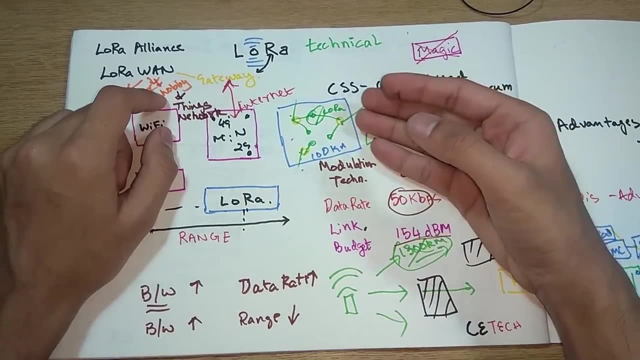 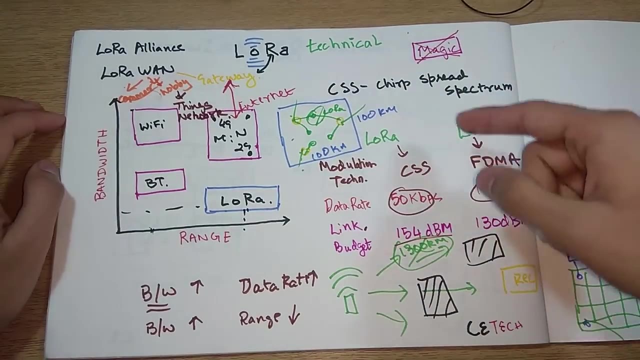 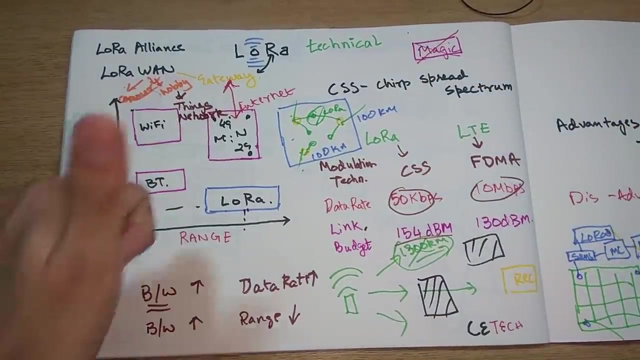 So, using the things network, you can use LoRaWAN to transfer data to your products. You can access a LoRaWAN gateway. All the people- general public- have their gateways installed. You can send data to their gateways and vice versa. You can also set your gateways. I recommend you do that so that you also contribute to the community. That is important to make the things network a successful platform. 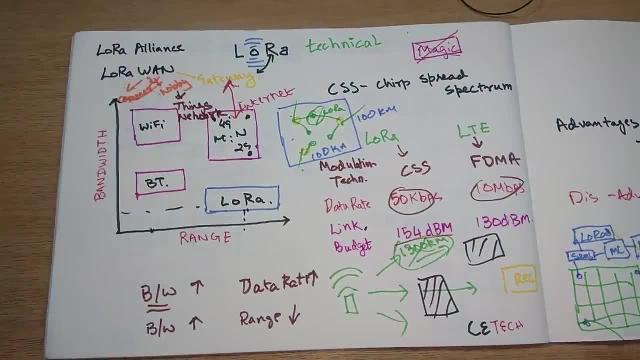 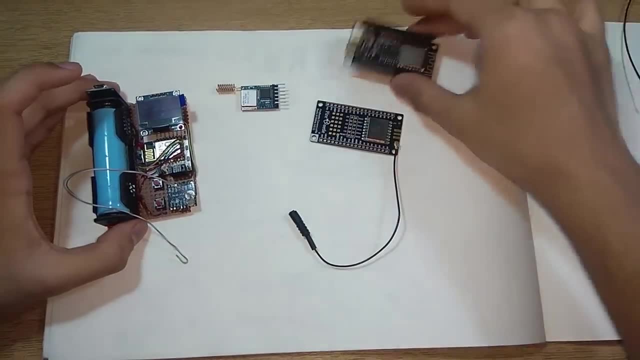 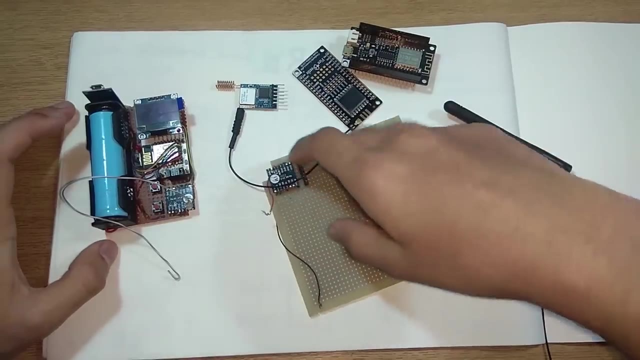 Things network is also a part of LoRa Alliance. So now moving from the technical part to the interesting hardware. So there are many modules that you can purchase. I'll mention all the links in the description below which you should, which you can buy to get started. 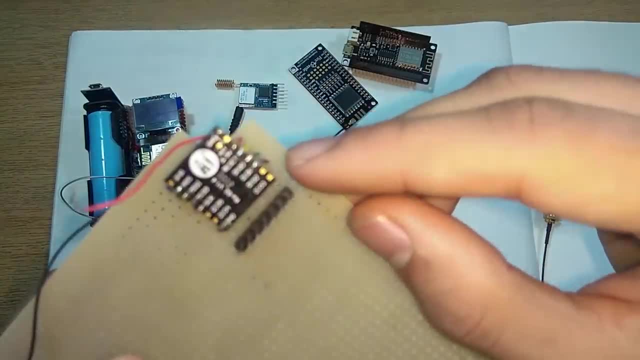 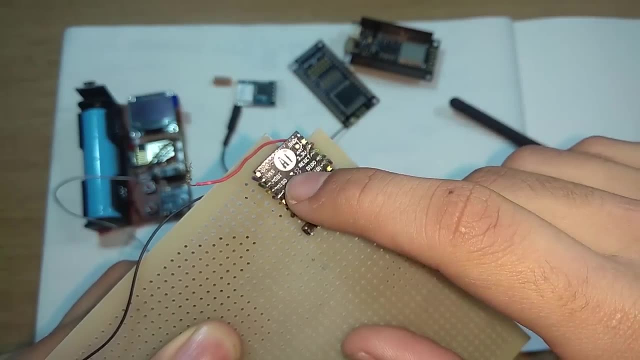 So this is the basic module. I've done it upside down because it was an SMD part and I had to solder it on a perf board. So this is a RA2, RA02, which consists of a Semtech SX1768, if I'm not wrong. 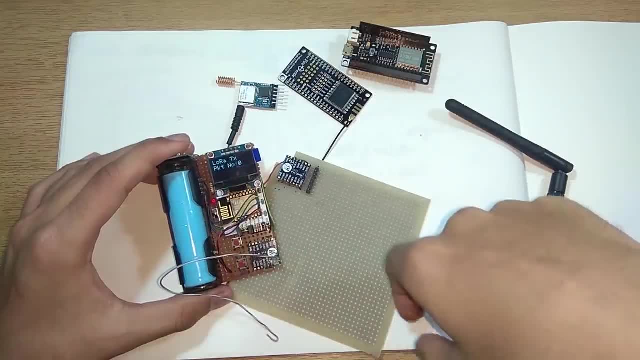 And I've made a project also. So this is a basic LoRa And this is a LoRa transmitter module which sends out packet. And this was my first project, So I didn't even use a proper antenna, I just used a wire. 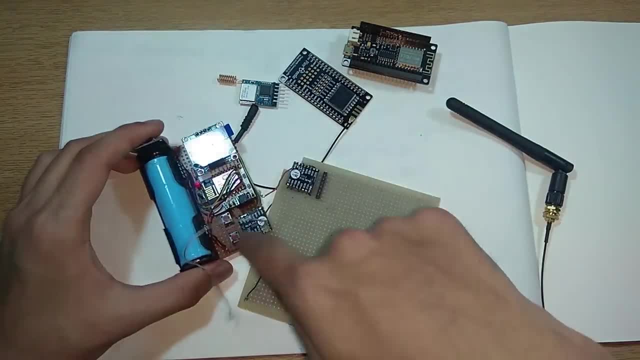 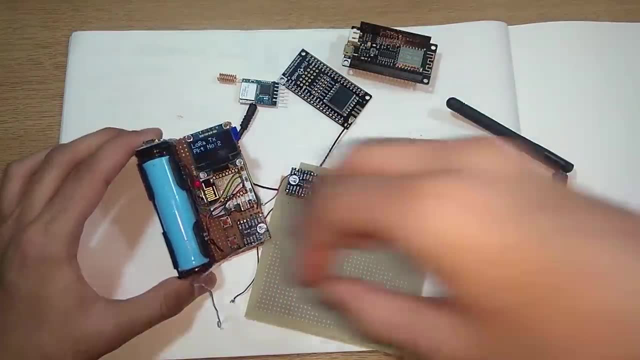 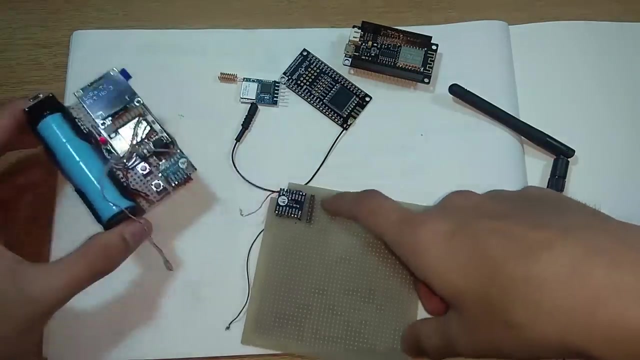 And it still works perfectly fine. So it has an OLED display, a battery, a LoRa module, an ESP8266, and it just transfers packets to a range around 8. And that is a LoRa transmitter. We'll make this on our channel. Stay tuned to our channel. 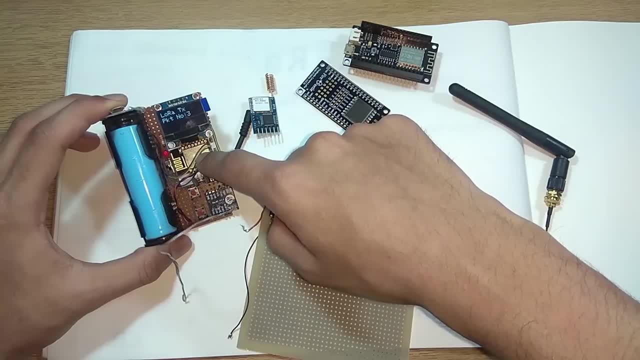 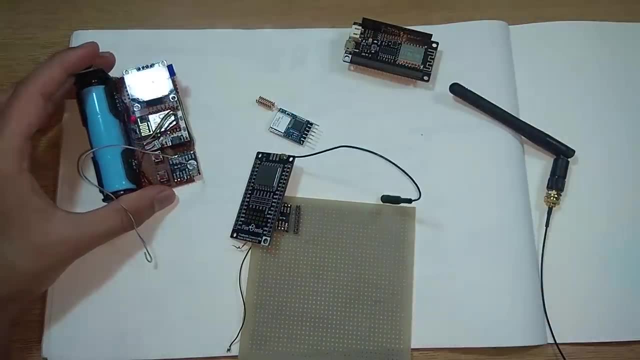 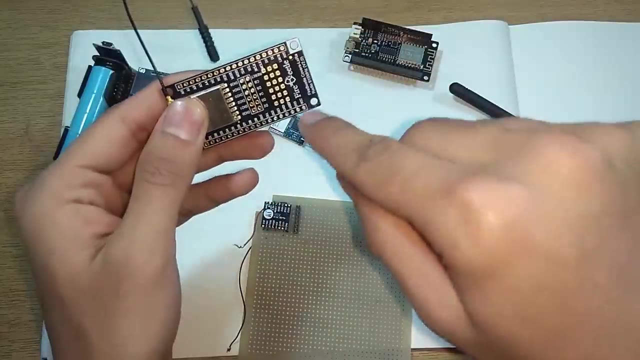 Other module is. so this module is connected to the ESP8266.. ESP8266 using an SPI MOSIMI, so SCK pins, similar. this one is for 433 megahertz frequency and the RA02. I bought this module, which is the 915 megahertz module from DF robot and this is a 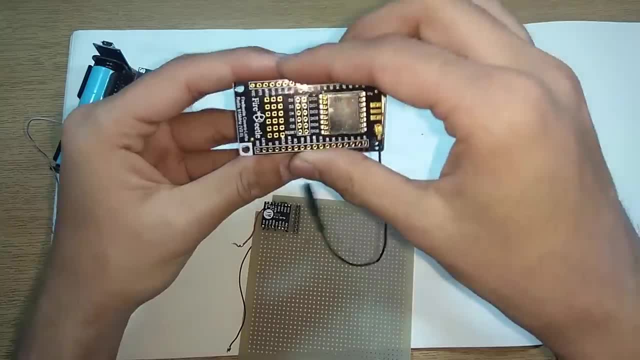 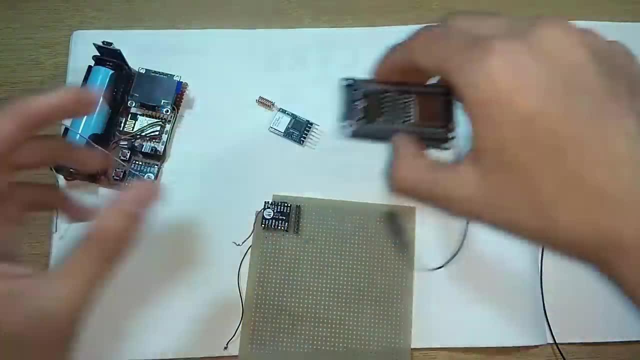 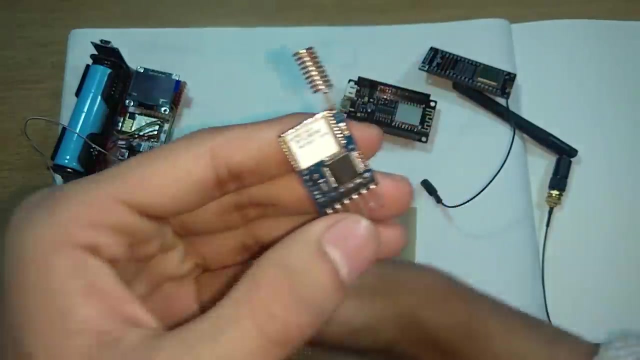 fire beetle series, so you can just solder pins and plug it in on an ESP8266- very useful if you are not into soldering and stuff. we will do a video on this as well. and this is the LoRa module. again, this is the 890 megahertz frequency module and this has a microcontroller built in, so you 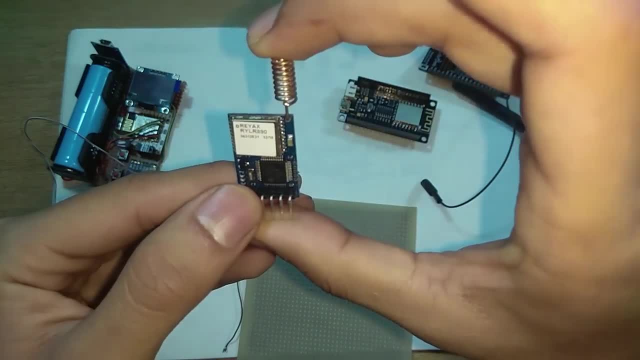 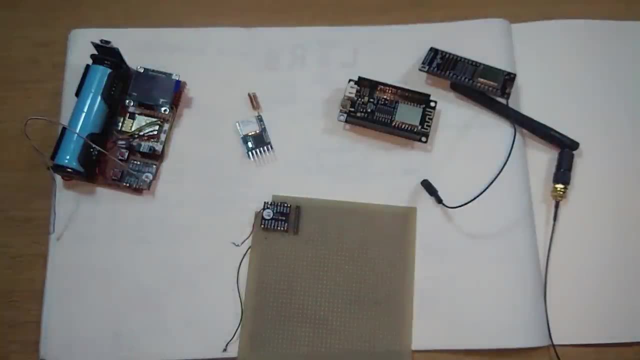 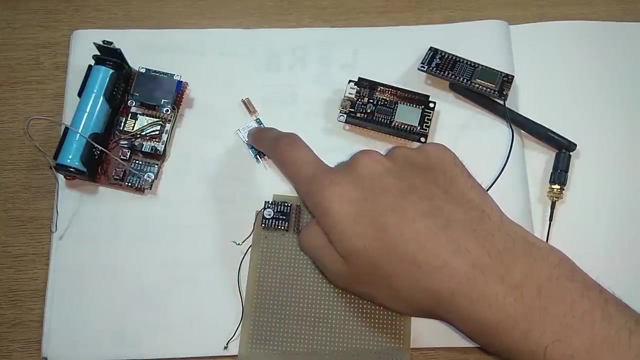 can use this directly as a UART device. so there is RX and TX pins, which directly sends in data etc. so you can control this device using AT commands. this is a device from, this is a module from reacts. I will mention both the links for the fire beetle from DF robot and.